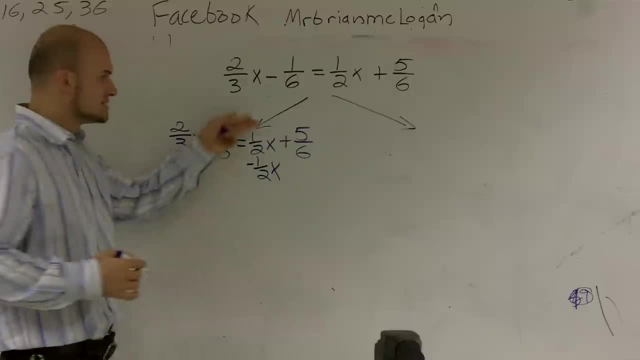 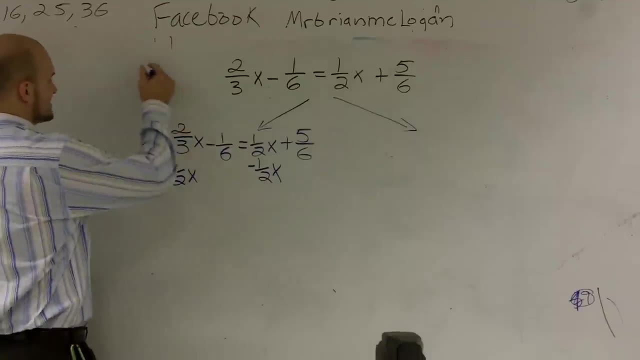 So I'm going to subtract my 1 half x. What that's going to do is that's going to get rid of my variable on the right side. Now why this is not a very preferred method is students hate subtracting fractions? It's not. 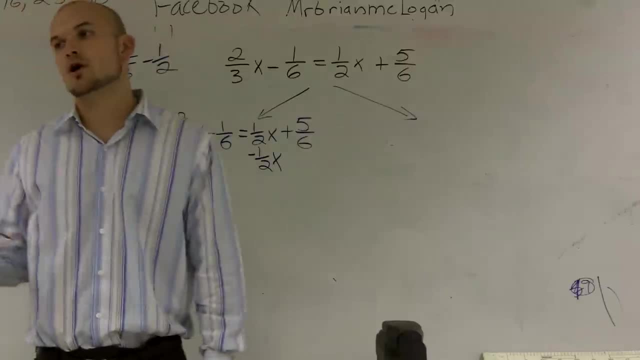 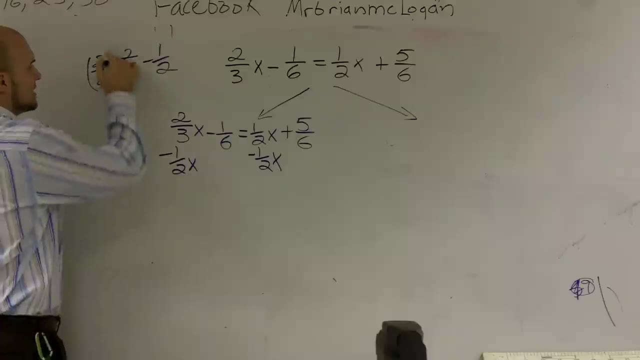 All right, But you guys need to know the process of subtracting fractions. These do not have the same denominator, So I need to multiply the left by 2 over 2 and the right by 3 over 3, because the least common multiple of 2 and 3 is 6.. 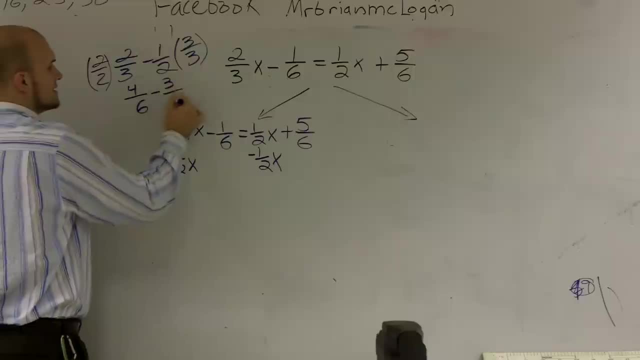 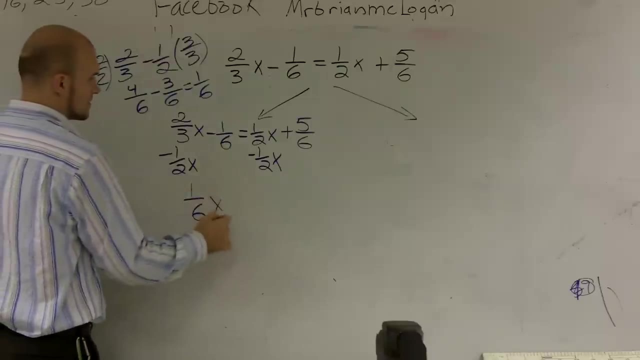 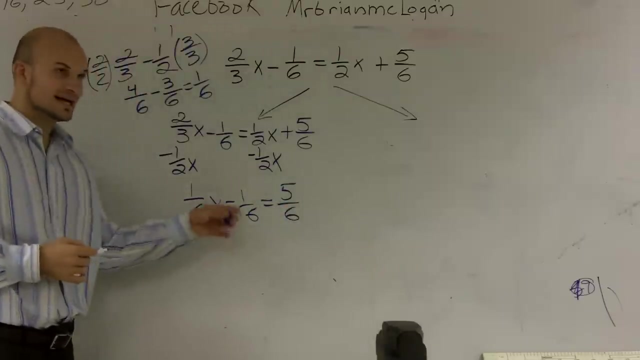 So therefore, I'm left with 4 sixths minus 3 sixths, which equals 1 sixth. So therefore, this is 1 sixth x minus 1 sixth. This is 1 sixth equals 5 sixths. All right, Then I need to get this fraction. 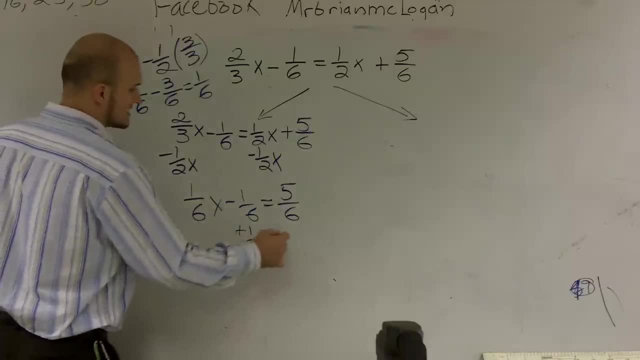 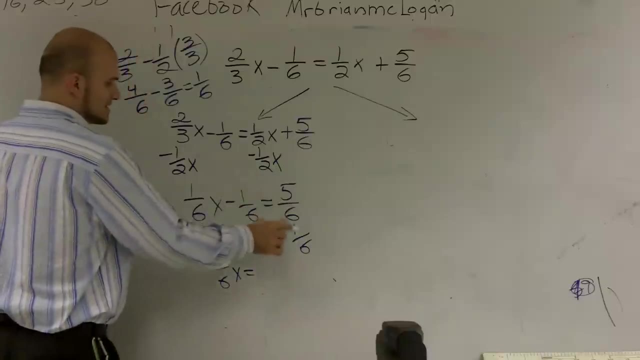 I need to get rid of this fraction, So I need to add 1 sixth on the both sides. So therefore I have 1 sixth x equals 5 sixths plus 6 sixths is going to give me 6 sixths, which is equal to 1, right. 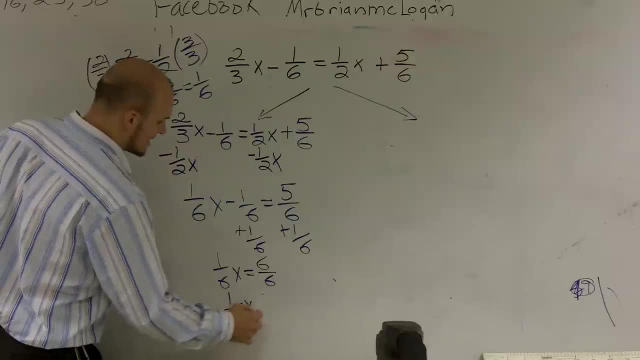 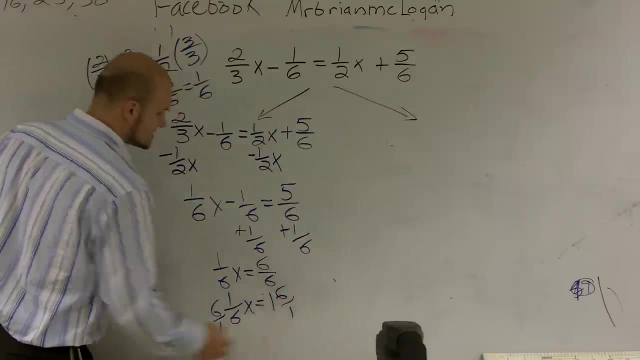 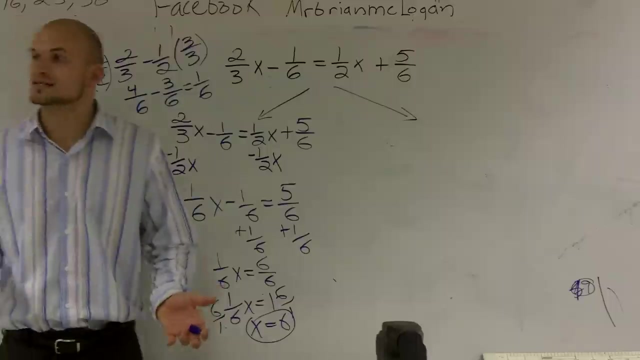 So now what I really have is: I have 1 sixth, x equals 1.. To get rid of this fraction, I can multiply by the reciprocal on both sides, And what I obtain is x is equal to 6.. Now let's check it another way to see if we're going to get the same answer. 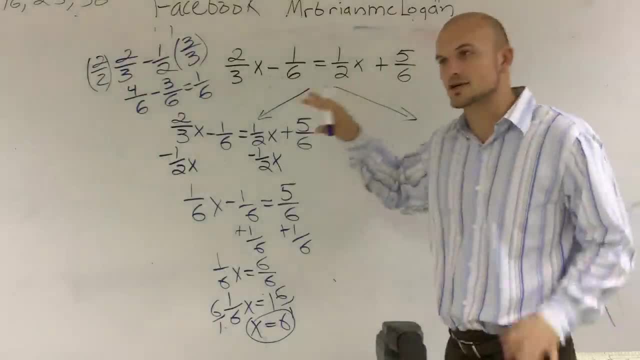 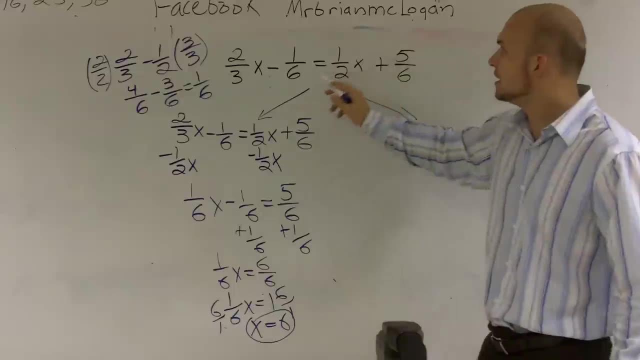 A lot of times. what I don't like to do is: a lot of you guys are going to hate fractions, right? So you won't even want to attempt this. That's fine, That's okay. What you can also do is get rid of all these fractions. 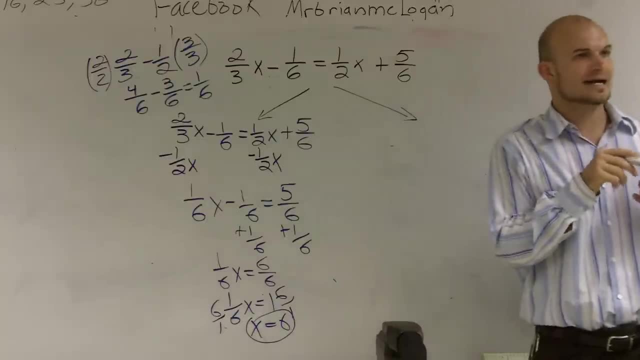 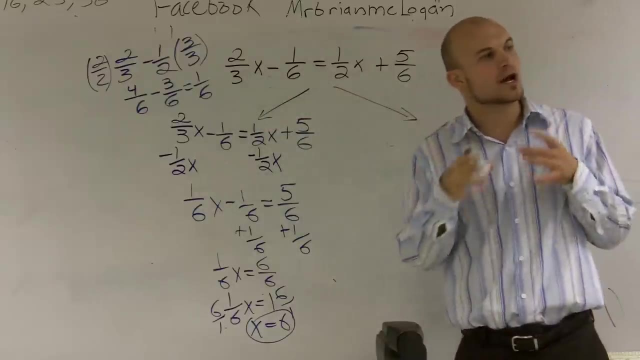 So what you want to do is you want to multiply by Multiply by the least common multiple of all your denominators. So if I look at here, I have 3,, 6,, 2, and 6.. So what is the smallest number that all those numbers go into? 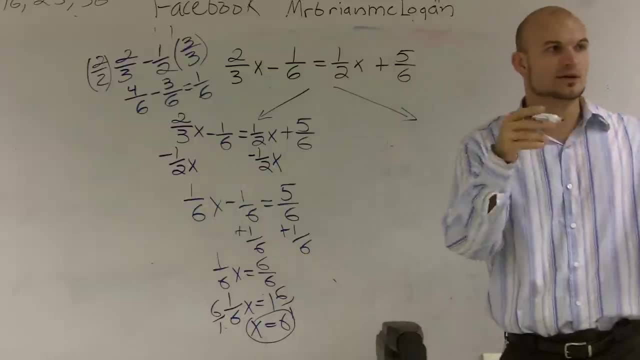 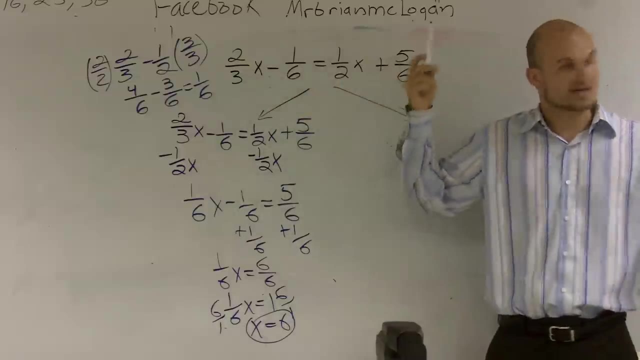 Yes, 2.. Oh, not the smallest number that goes in, What's the smallest number that all of these go into, Like what's the least multiple of all those 6. 6, exactly. So, therefore, what I get is: so, if I do 2 thirds, 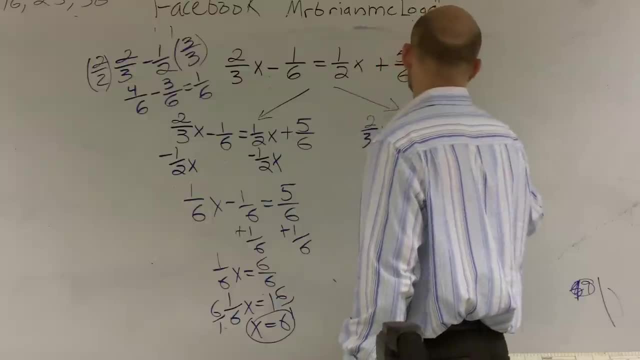 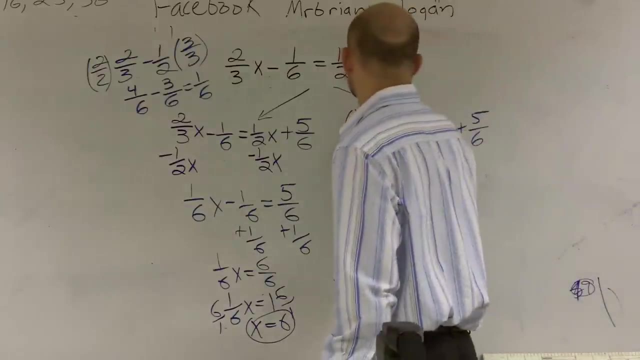 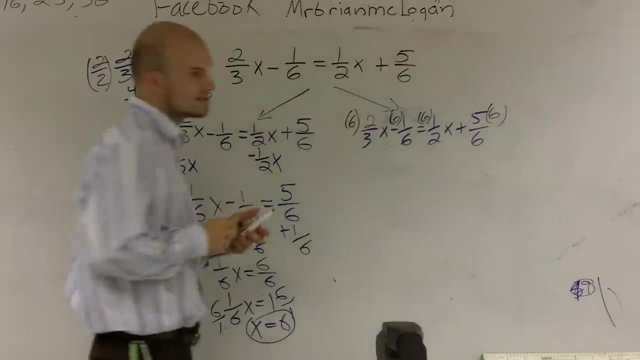 x minus 1 sixth equals 1 half Half x plus 5 sixths. So if I'm going to multiply, I'm going to multiply everything by 6.. You really have to pay attention to this, because this is where a lot of you are going to make your mistakes. 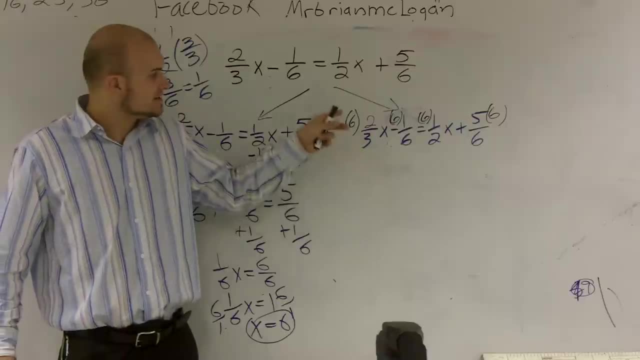 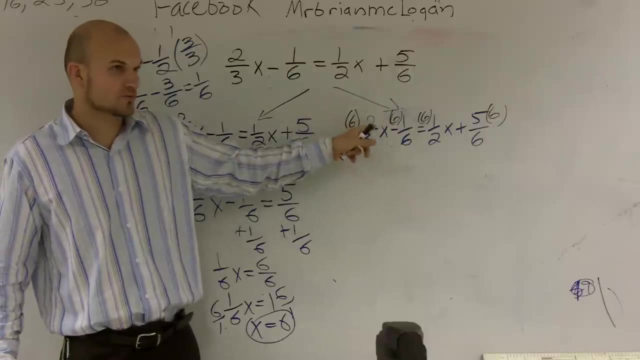 You have a number on the numerator and you're going to have a number on the denominator. okay, 6 divided by 3 gives you what 2.. 2 times that 2 is what 4., 4., 4.. 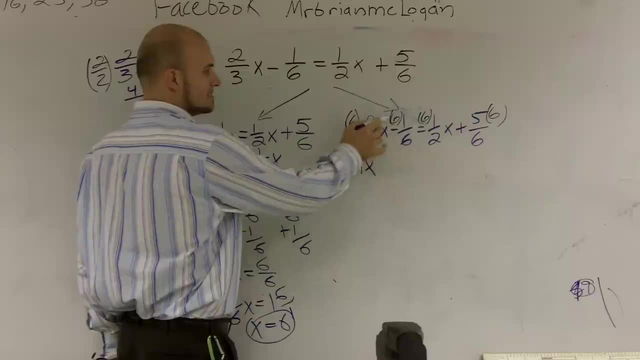 6 divided by 6 is 1.. 1 times this negative 1 is 1.. 6 divided by 2 is 3.. 3. 3 times 1 is 3x, 3x. 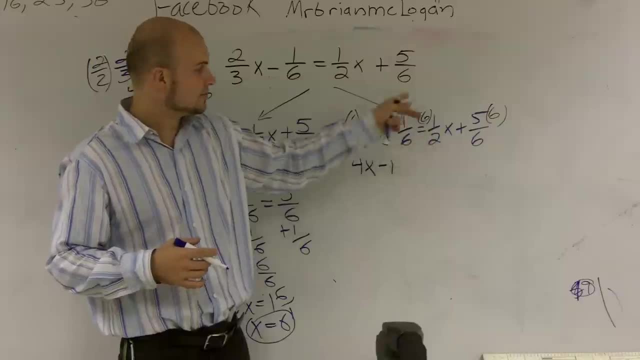 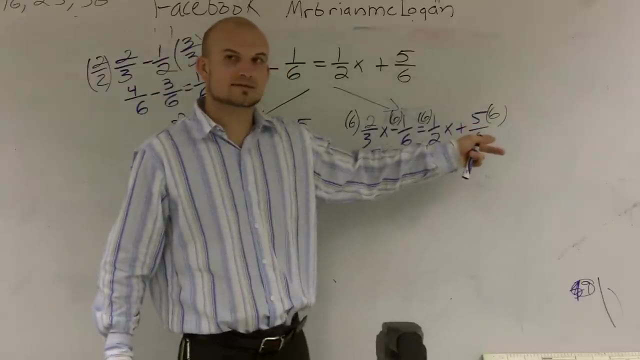 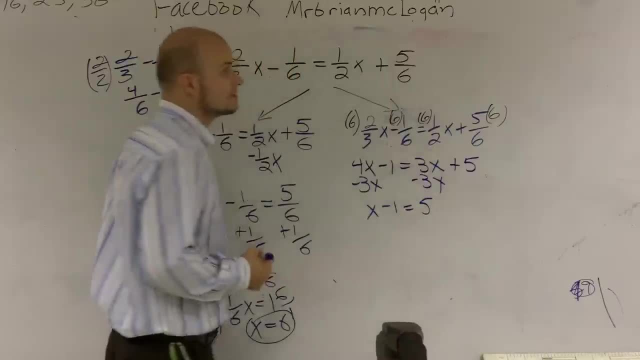 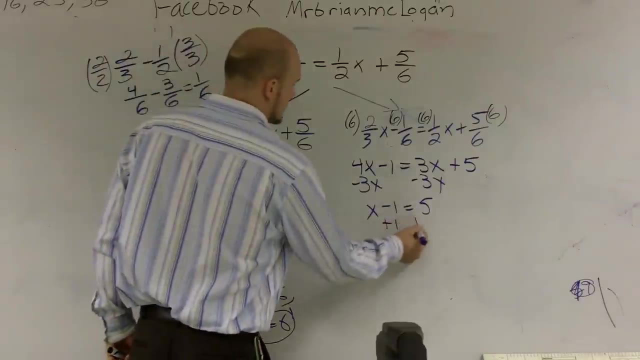 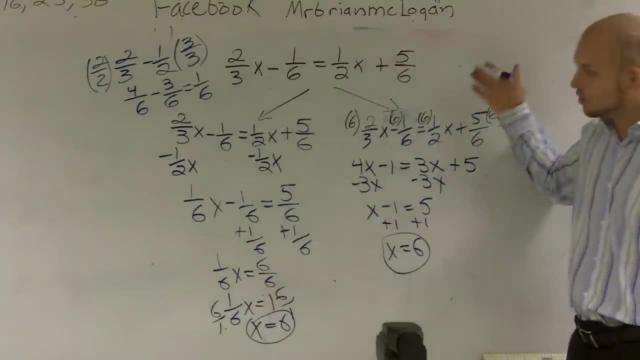 which way you want to do it. You can either solve it with fractions or you can get rid of everything by multiplying by your all these kind of multiples, And that's how you solve when you have a variable on both sides, with fractions. 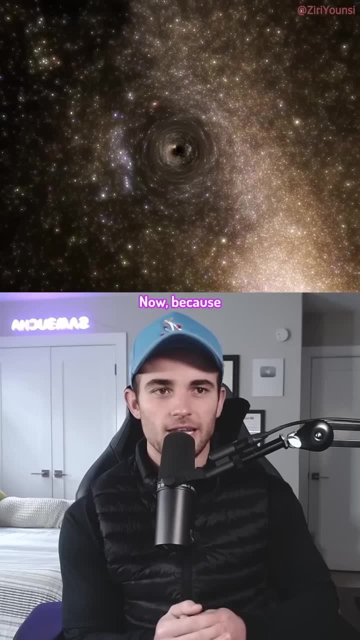 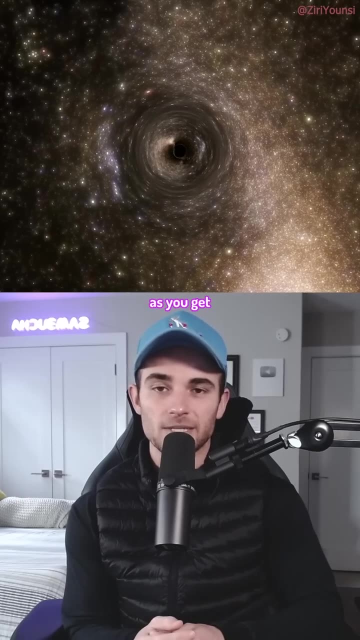 Here's what it would look like if you were falling into a black hole Now, because a black hole is infinitely dense and all matter is concentrated in the point of singularity at the center. you'll actually speed up as you get closer and closer to this beast.